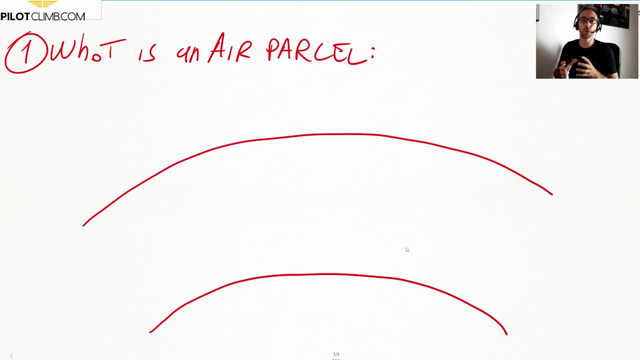 they don't okay. But how come that the an air parcel has got different characteristics compared to the air surrounds? okay, let me give you an example. So if you look at the whiteboard in here we've got, let's say, this part of here, okay, this part of here is sea, okay. so you've got water in. 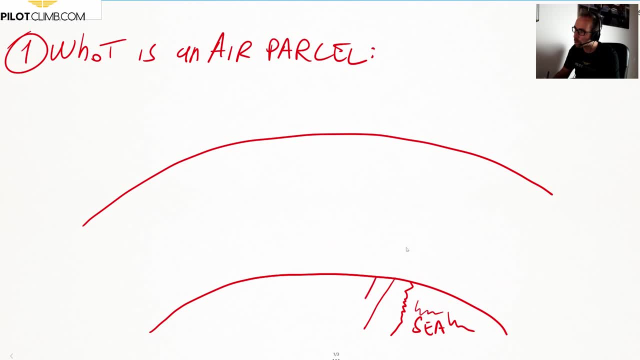 here and in next to the sea, you've got a road, so you've got some asphalt, okay, and, as you know, the asphalt actually warm-ups quicker than the sea. so the asphalt, because of the characteristic of the asphalt, warm up quicker than the water. all right, So what will happen is that if I make 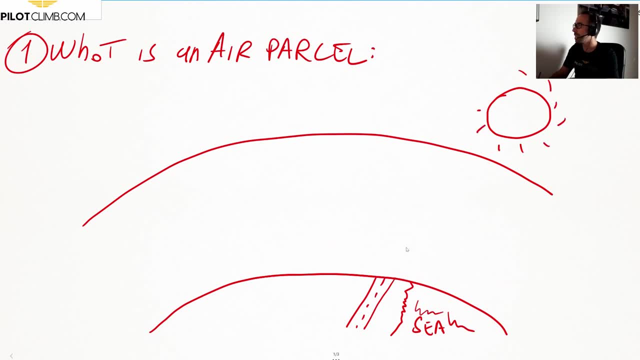 if I draw a nice sun in here, guys- okay, this is the nice sun- what will happen is that this sun will actually warm up the earth's surface. okay, with these radiations, okay so. and then what will happen is that the asphalt part, okay the road, will be warmer than the sea. thus, the asphalt will warm up the. 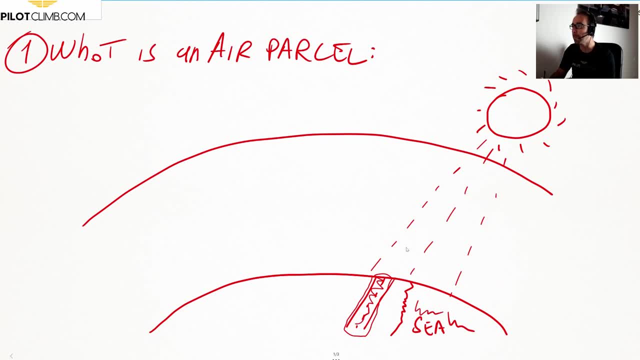 air that is on top of the asphalt will be warmer compared to the air that is on top of the sea. okay, So, as you can see already, the air on top, the mass of air, the parcel of air that is on top of the asphalt will be warmer compared to the mass of air that is on top. 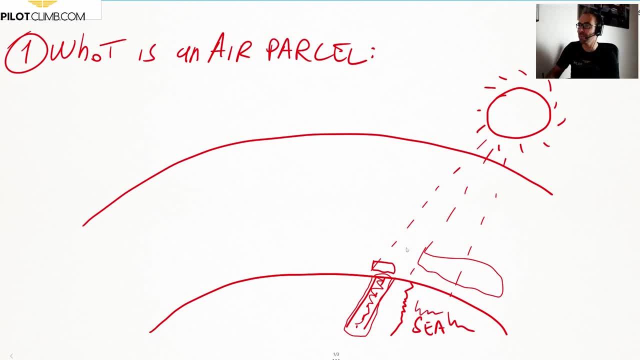 of the sea. so, as you can see, already we've got the environmental air, that is, the atmospheric air, and then we've got this: a parcel of air on top of this road and a parcel of air on top of the sea. as you can see, the atmosphere is composed by multiple parts of air, and then you've got the 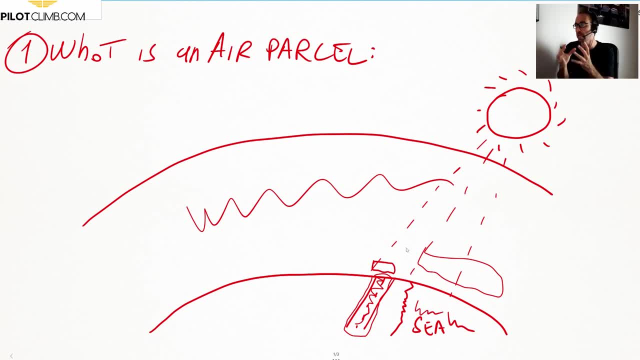 environmental. so you need to understand how can you actually differentiate between the environment and the air. so this is the parcel of air. the mass of air, as we said, on top of the asphalt will be warmer. thus, when something is warmer, when a mass of air is warmer than environmental air, what will? 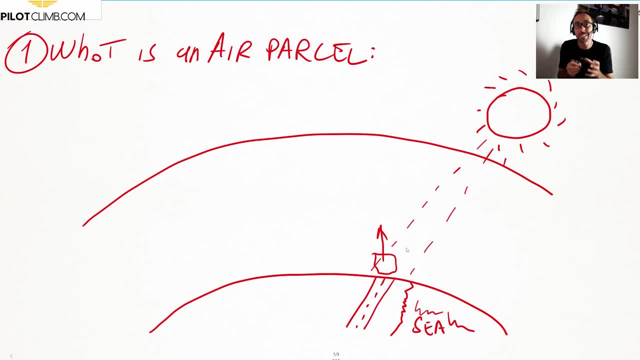 happen is that it will start to rise, because being being warmer means being less dense, thus being lighter than the environmental air. thus, if this parcel of air is lighter than the environmental air that is around will start to rise. okay, So this is a very basic concept we need to understand in order to make sure we get in full the environmental lapse. 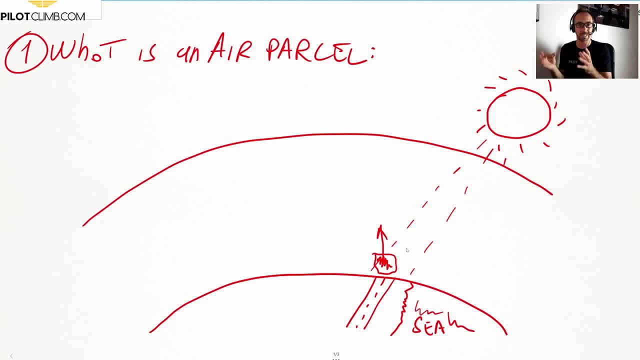 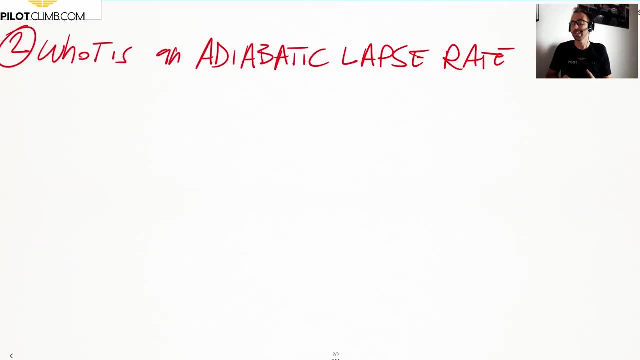 rate, the saturated lapse rate and the dry adiabatic lapse rate. all right, so let's move on. if i go on the slide number two in here, it says what is an adiabatic lapse rate? so the ad, the lapse rate, is the change in temperature with your height. okay, so the standard environmental. 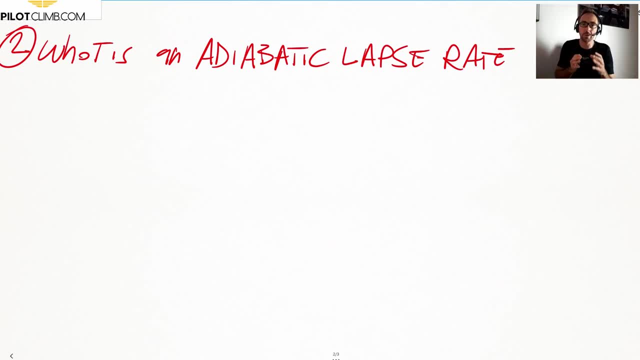 lapse rate, according to the standard atmosphere is two degrees per 1000 feet. what does it mean? so if this is the sea level, okay, according to the standard atmosphere, the temperature at the sea level is 15 degrees celsius, okay, and the lapse rate is two degrees per 1000 feet. so if we've got, 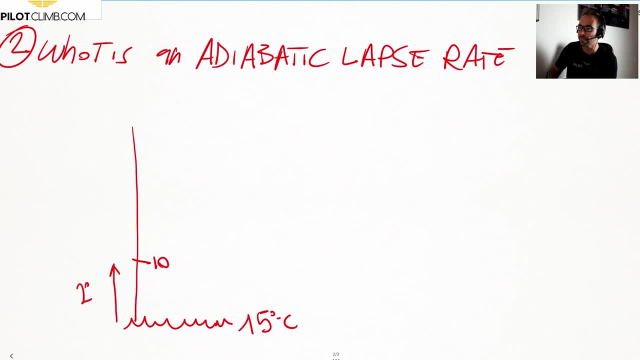 15 degrees celsius at the sea level at 1000 feet of height or altitude. in this case, we can say that the temperature will be 13 degrees celsius. at 2000 feet, the temperature will decrease by another two degrees. does we're gonna? we're gonna have 11 degrees celsius? so the lapse rate is the change. in temperature, with your altitude, with your height. okay, so every 1000 feet you have a lapse rate of 2 degrees. that means the environmental lapse rate according to the standard atmosphere is 2 degrees every 1000 feet. this is the standard atmosphere. guys, we need to understand in real life this is. 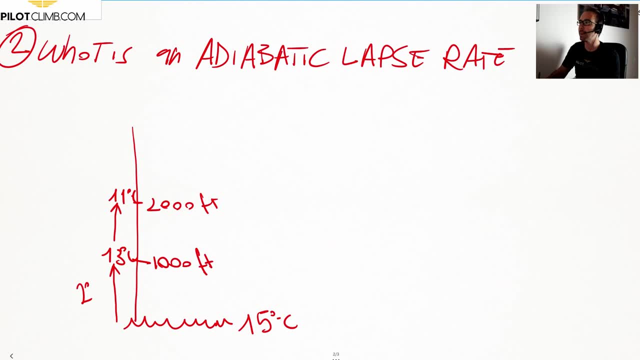 not always the same in real life. this is a standard very nice, but, however, in real life, the temperature- not 15 degrees- can be 5 degrees, for example, or 30 degrees. it really changed by the day by day and the environmental lapse rate. okay, the, the the temperature change with the, with the, with. 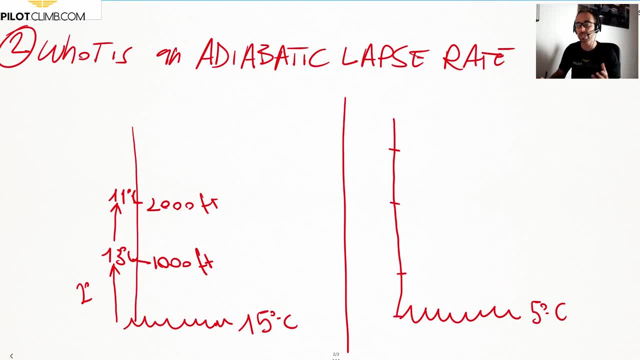 the altitude doesn't stay constant by two degrees every one thousand feet. it may be one day five degrees, or one day maybe one degree, so it really depends. so then, once we understand what is the environmental lapse rates, the standard one which is two degrees per one thousand feet, and we 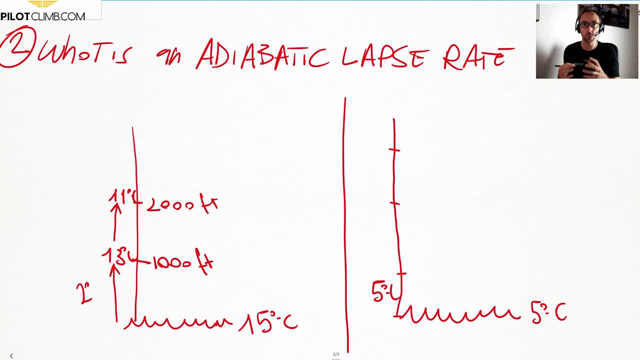 understand that this is a standard. in the real life, the things can change. we actually get into the atmospheric stability, okay, then we're gonna have one day atmospheric stability. one day we're gonna have us atmospheric instability, but we're gonna talk about that in a in a later video. okay, 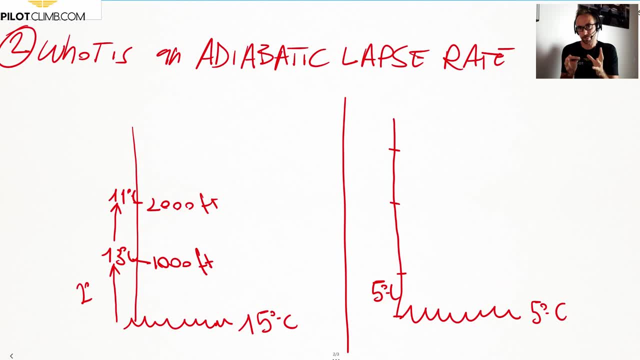 so beautiful. what is an adiabatic lapse rate? all right, so let's take the example that we made before. so let's say that we've got this c in here, and then, as we said, we've got our roads in here, okay. so, we've got, this is the road, okay. so, as we said, 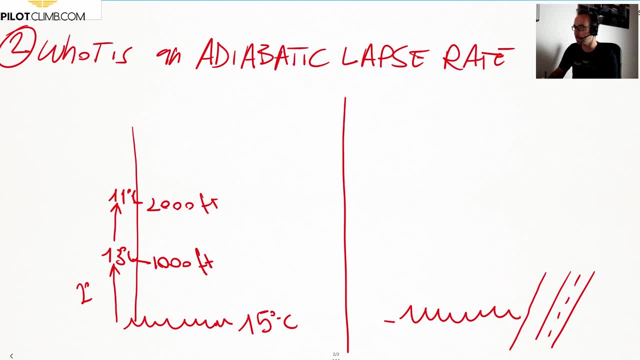 the air on top of the asphalt will be warmer. okay, thus, being warmer, that means that the the mass of air is actually lighter. thus this mass over will start to rise. okay, so, by adiabatic lapse rate means that this mass over, as it climbs, will became cooler. why? because 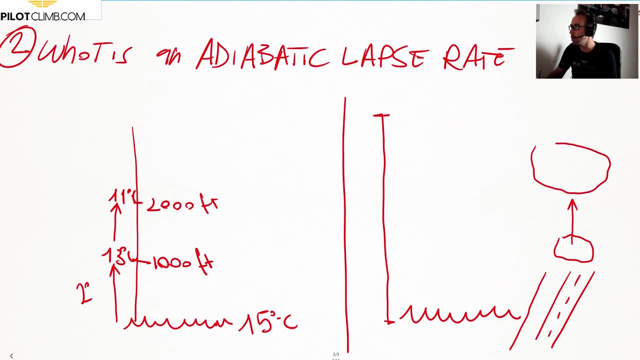 with the altitude, the mass of a will start to expand because there will be less pressure. thus by expanding is decreasing its temperature. however, there is not an exchange in any heat energy, so we are not actually cooling down by putting some ice in the in the air mass. this air mass is: 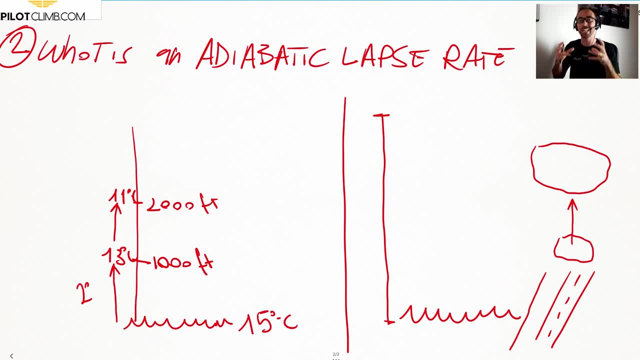 cooling down because it is actually expanding, and that means adiabatic, because we don't have any heat exchange- okay, we don't have any energy exchange between the air mass and the atmospheric and the environment, okay. thus, what will happen is that the molecular inside this mass of air, that is, that has 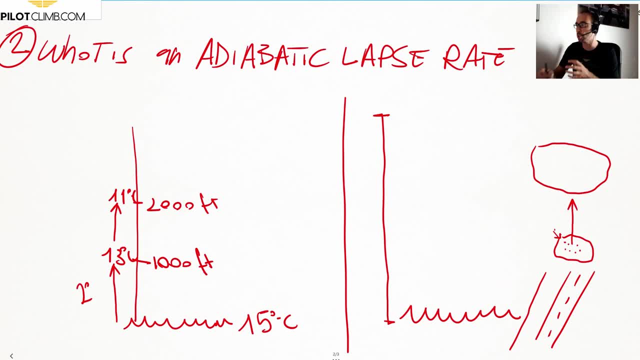 got this size in here, will move because they have a temperature. but by expounding, expanding this mass of air gonna give more room to this molecular to move. thus this molecular will start to move slower because they have more space and thus, by moving slower, the temperature will start to. 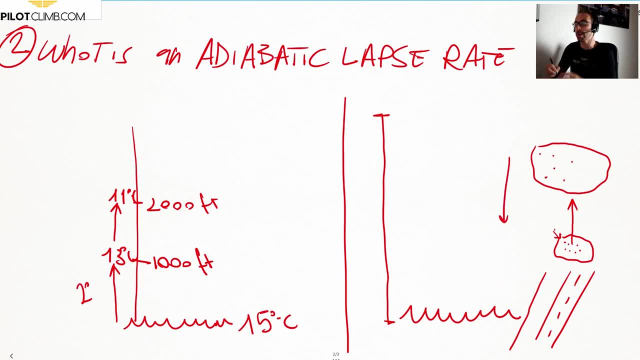 decrease. the same is true by when they hear another- and i must actually warm up at the batik. that means there is no energy exchange. it warm us because it goes from this size okay to this size, thus the molecular will will get. we get in a smaller place, thus they start to increase. 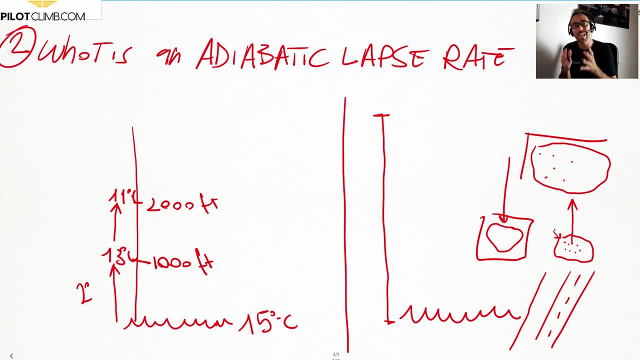 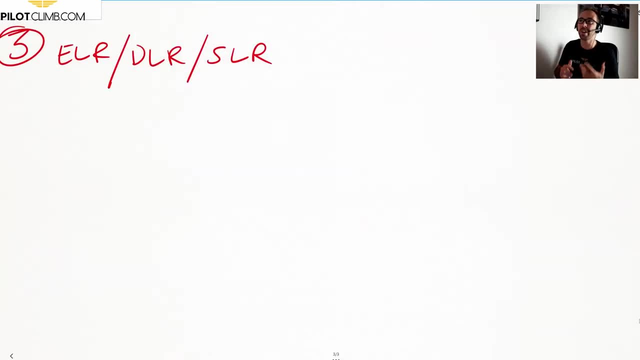 their speed. by increasing the speed, they will increase the temperature. this is called adiabatic lapse rate. okay, so this is very important to understand. now the last thing, in order to understand: what is an environmental lapse rate, what is a dry lapse rate? what is a saturated lapse rate? 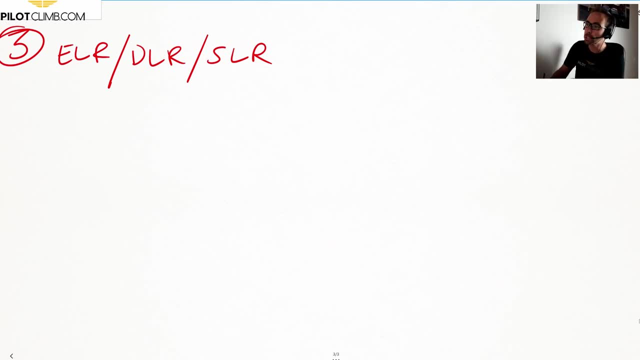 draw a, draw down a graphic in here, okay, so let's call it the standard, uh, lapse rate. okay, this is the c. okay, let me do the c and the road. okay, so we keep the example as before. so every thousand feet, guys, we've got two degrees according to the standard atmosphere. so this is zero, this is. 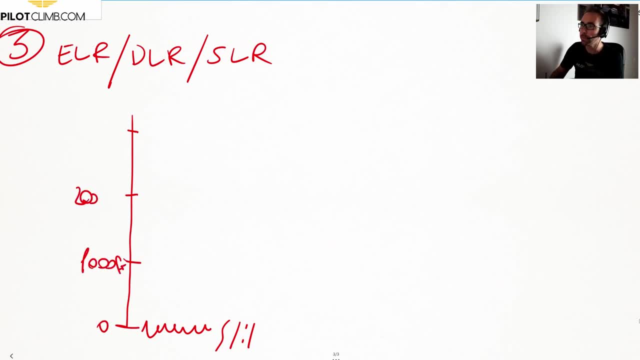 one thousand feet. okay, this is two thousand feet, all right, and this is three thousand feet, okay. so this is crucial to understand the topic, okay, so at the sea level, okay, we're gonna put in here the temperature. okay, the sea level is 15 degrees celsius at one thousand feet, we've got, uh, two degrees less, so will be 30 degrees, 13 degrees. 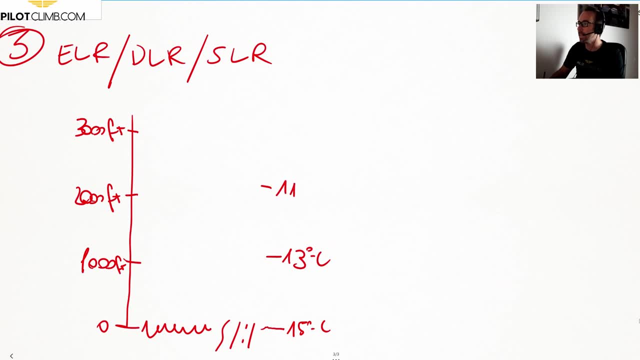 celsius to the uh, two thousand feet, we're gonna have 11 degrees celsius and then at three thousand feet, we're gonna have nine degrees. so this is according to standard, because the environmental lapse rate according to standard is two degrees. okay, now the dry adiabatic lapse rate. let's say: 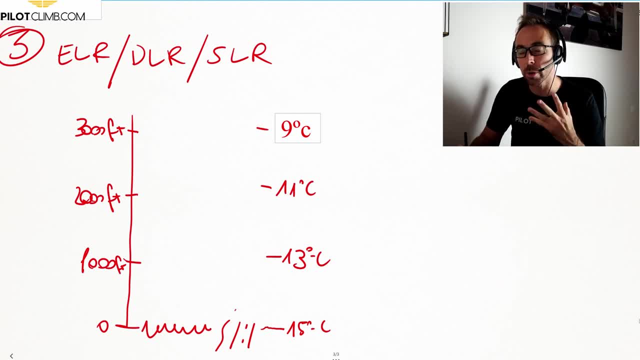 the air is going up the air. we've got an air mass on top of the asphalt. it is warmer, okay, and it's dry okay, because it's not condensated yet. it's not a cloud, it's just an air mass. it's just a bubble, okay, an air parcel, okay. since it's a dry, is a dry will start to rise and when you've 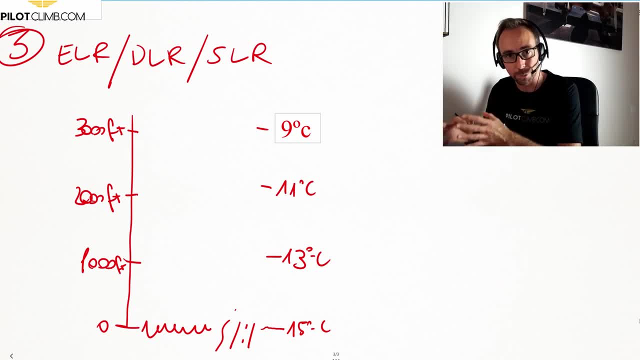 got an air pass that has got a dry adiabatic lapse rate. this dry adiabatic lapse rate will be a quicker than the environmental lapse rate, okay, so, as you can see, the air in the atmosphere will environmental lapse rate. however, the mass of air, because of its characteristics, gonna have. 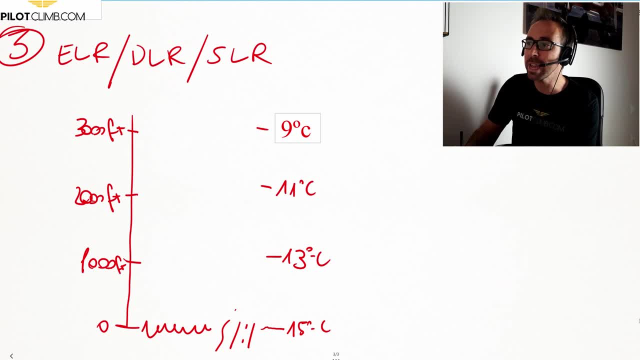 firstly, a dry adiabatic lapse rate. and this dry adiabatic lapse rate normally is not two degrees every one thousand feet but is an higher lapse rate. thus, if the mass of air at the mince level is 17 degrees, because it's warmer, because the the sun warm up the asphalt and the asphalt warm up. 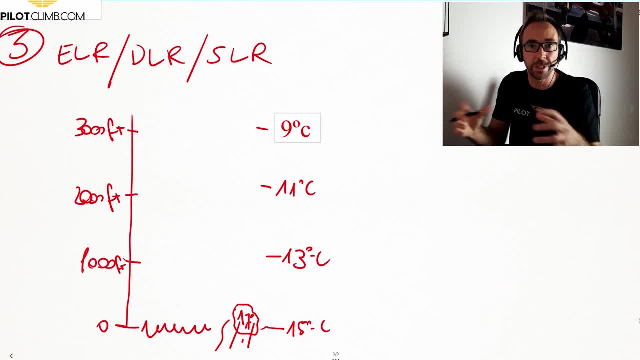 the air on top of the asphalt more than the air around the, the atmosphere air, this mass of air will start to rise and and will decrease its temperature using the dry adiabatic lapse rate. let's say the dry adiabatic lapse rate will be three degrees per one thousand feet. 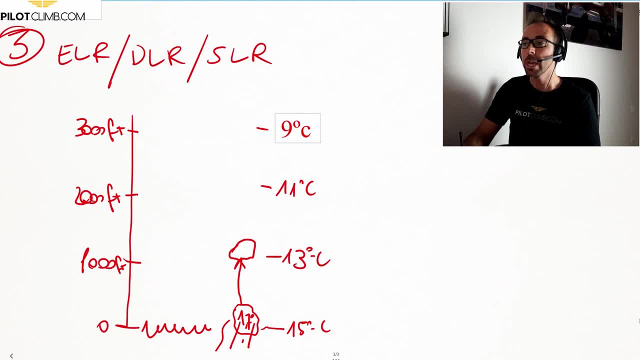 thus, once the mass of air reach the one thousand feet, it will have 14 degrees and not 13 degrees, because by one thousand feet it decreases three degrees and not two degrees. okay, then, at two thousand feet, if we keep climbing, okay, this mass of air is going to have 11 degrees and, as you, 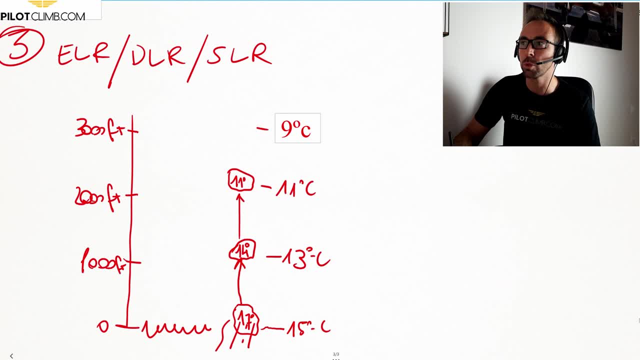 can see, once this mass of air gets to this point- 2000 feet in this example- the mass of air will stop to rise. you may ask: why is because, as we said before, if an an air parcel is warmer than the surrounding air, it will rise because it's lighter. thus, in in the first case, on the missy level, that parcel of air was 17 degrees and the outside temperature was 15,. thus the parcel of air is warmer, so it will start to rise On 1,000 feet. the environmental air temperature was at 13 degrees. however, the parcel of air was 14,, still warmer. thus it will keep rising. 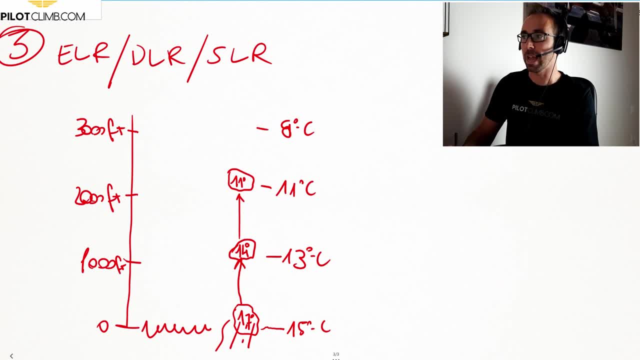 until it gets to the point where the environmental air temperature and its temperature of the parcel of air is the same, and then it stops. Okay, so, as you can see, we actually put. now we've got this is the environmental lapse rate, which we can call it 2 degrees per 1,000 feet. okay, 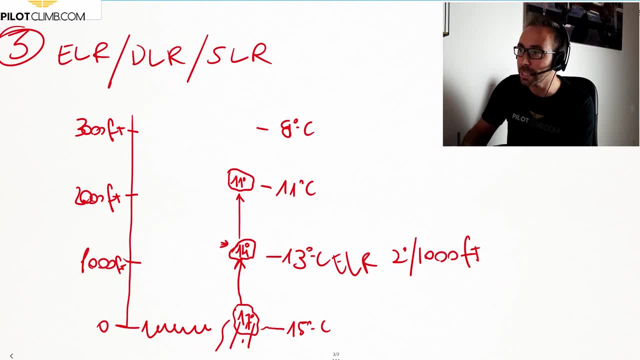 according to standard and this is the dry. in this case, this is the dry, which we said is 3 degrees per 1,000 feet. So, as you can see, we have got two different lapse rates: one is the environmental and the other one is the dry adiabatic lapse rate. all right. 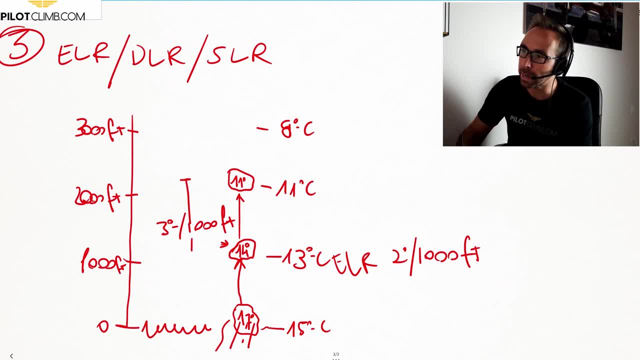 Beautiful. So from this part to this part: okay, the mass of air climbed using the dry lapse rate. okay. so in this part in here, However, let's say that the mass of air has got some moisture inside. okay, will reach a point where it starts to condensate. okay, 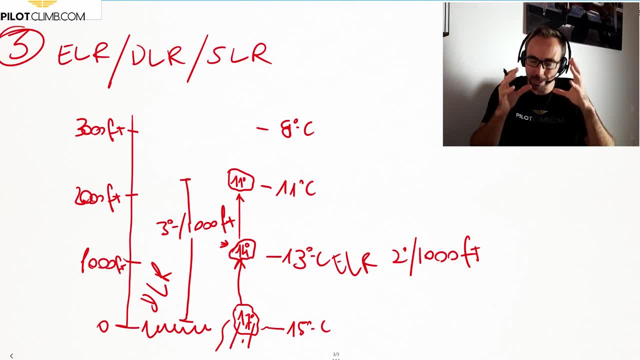 This point is called dew point. okay, When you actually, when the temperature of a mass of air reaches the dew point temperature, it will condense, because the mass of air won't be able anymore to, okay, sustain the water vapor. Thus it will condense, okay. 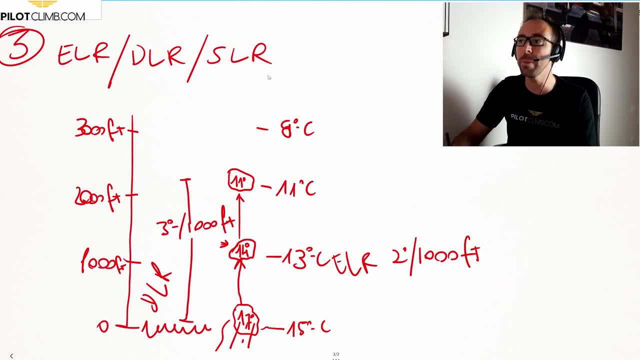 Once the mass of air will condense, okay, it becomes clouds. And once it becomes clouds, if the mass of air will keep rising, it will not have a dry adiabatic lapse rate, but it is going to have a saturated lapse rate, okay. 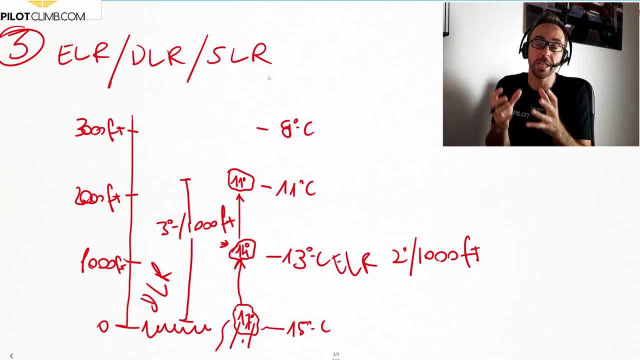 So the mass of air will decrease in temperature if it keeps rising. in this case it's going to be the clouds. the air inside the cloud will decrease in temperature following the saturated lapse rate. okay, Okay. So let me make another example in here. 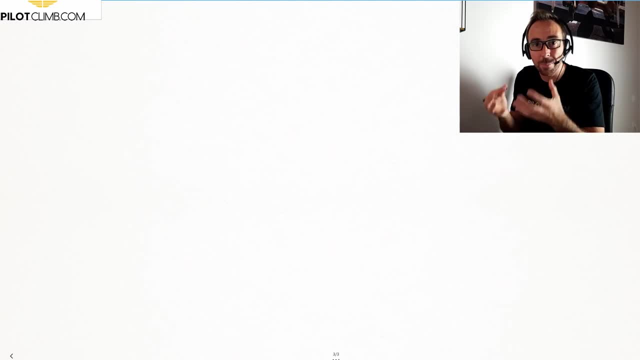 All right, guys. so let's see how a parcel of air will start climbing using the dry adiabatic lapse rate And then, once it reaches the dew point and the condensation, we'll start using the saturated lapse rate. OK, so let me give you an example here. 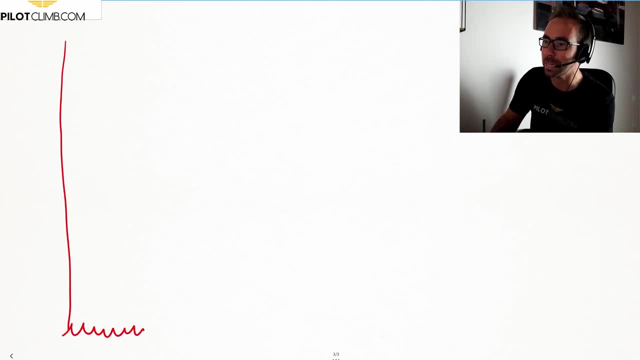 So I'm going to put an altitude scale in there. the mean sea level, That is 0 feet, That is 1,000 feet. OK, This is 2,000 feet, 2,000 feet, 3,000 feet in there. 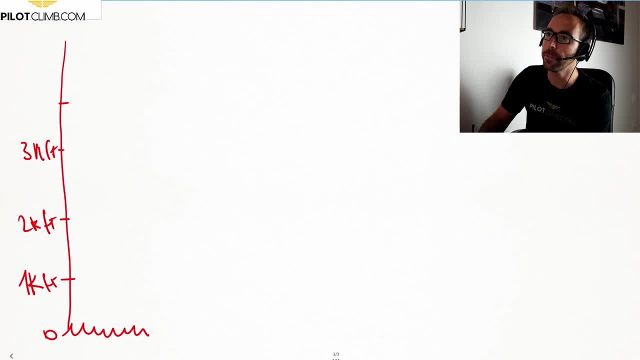 3,000 feet And 4,000 feet And 5,000 feet is in there, OK, All right. so 1,000 feet, 2,000 feet, 1,000 feet and so on. 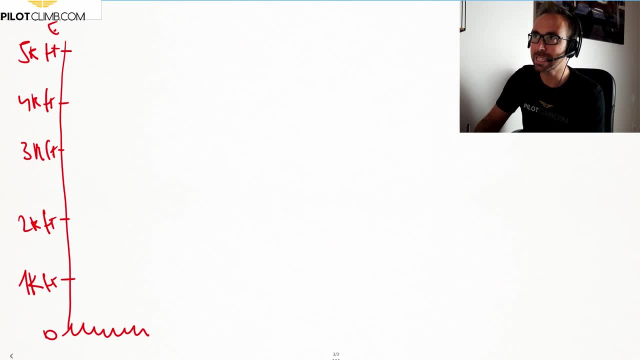 The environmental lapse rate. OK, the standard environmental lapse rate is 2 degrees per 1,000 feet. Thus the temperature of the mean sea level is going to be 15 degrees. So I can write down 15 degrees Celsius And 1,000 feet will be actually 2 degrees warm colder. 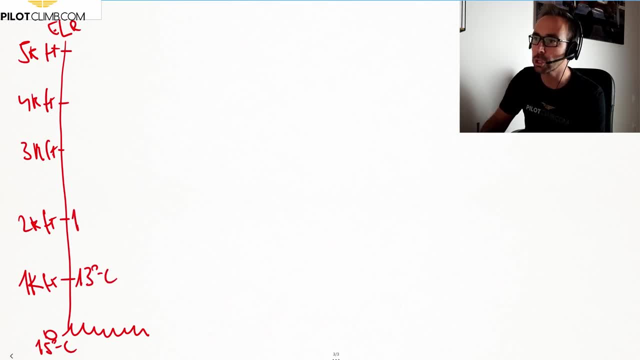 So that means there's going to be 13 degrees Celsius At 2,000 feet, it's going to be 11 degrees Celsius, And then it's going to be 8 degrees Celsius in here And 5,- sorry, 6- degrees Celsius. 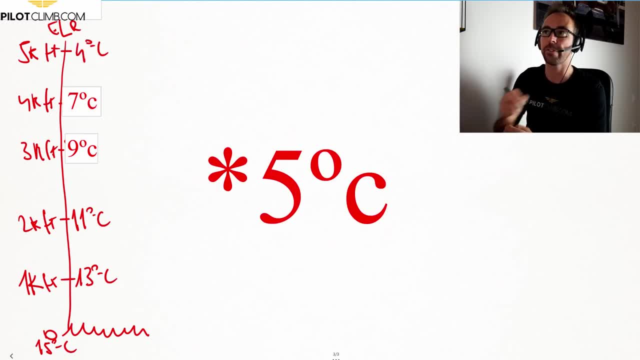 And then we're going to have, lastly, 4 degrees Celsius at 5,000 feet. This is the environmental lapse rate. the air: How does the temperature of the environmental air change with the height? OK, However, if we make the example that we did before with the roads, OK, let's say that the sun will actually warm up. 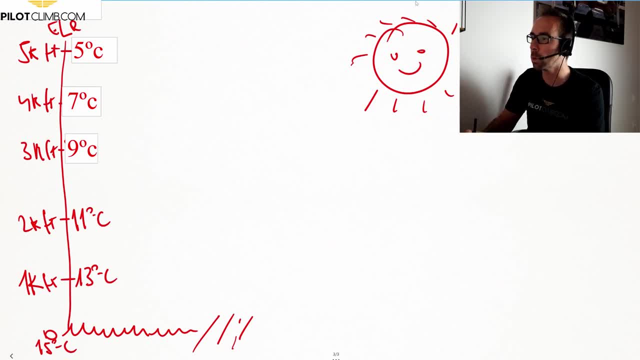 The roads, OK. so this is our nice sun that is warming up the roads, OK, And let's say that a parcel of air that is on top of the asphalt is warmer. Thus, let's say that this parcel of air will start with a temperature of 20 degrees Celsius because it's warmer, since the asphalt is warmer. OK, so let's say that the dry lapse rate of this parcel of air will be 3 degrees per 1,000 feet. OK, and let's say that it's saturated lapse rate, which we said is It's lower since we've got this condensation, is 1.5 degrees per 1,000 feet. all right, 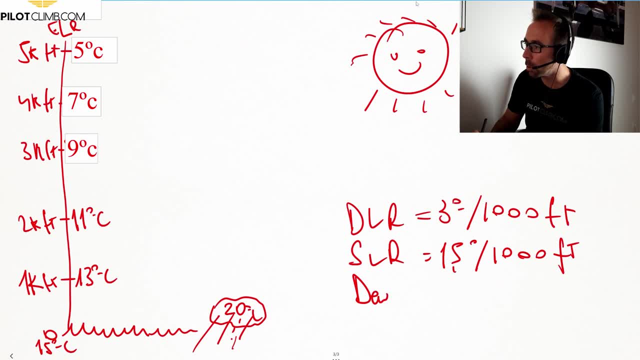 And lastly, let's say that the dew point of this mass of air it's going to be, let's call it, 15 degrees. OK, So now we know that that mass of air will, once it reaches the 15 degrees Celsius temperature, it will actually condensate because it reaches that dew point. all right, 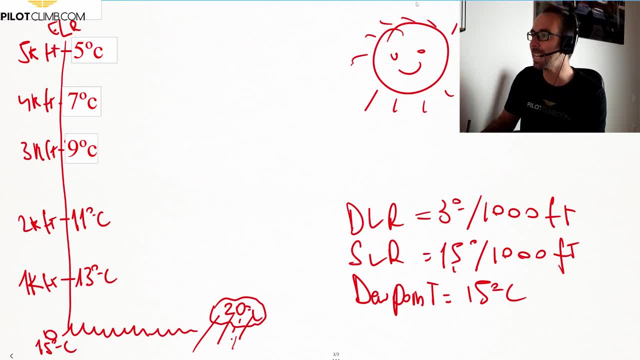 So let's say: Let's see how does it work. So, first of all, the sun will warm up the asphalt. OK, Thus the asphalt is going to have an higher temperature compared than the environmental air temperature. Thus the mass of air that is on top of the asphalt is actually warmer, lighter. 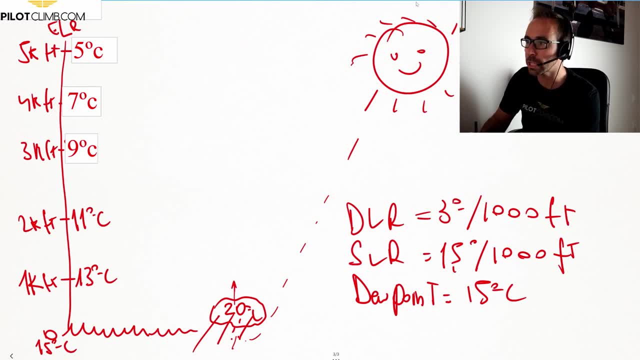 Thus it will climb, So it will get to its first 1,000 feet check mark. OK, The mass of air will be a little bit bigger because it's expanding, and at 1,000 feet will be at 17 degrees Celsius still warmer, OK, 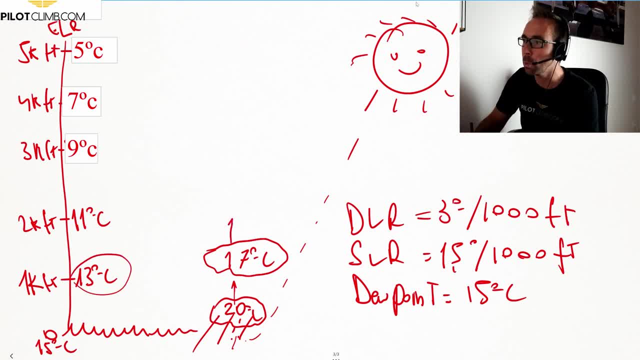 Compared to the Environmental air. So we'll keep rising. It will reach the 2,000 feet check mark, OK, And it will reach actually 14 degrees, OK, So fantastic. As you can see, it's still warmer. 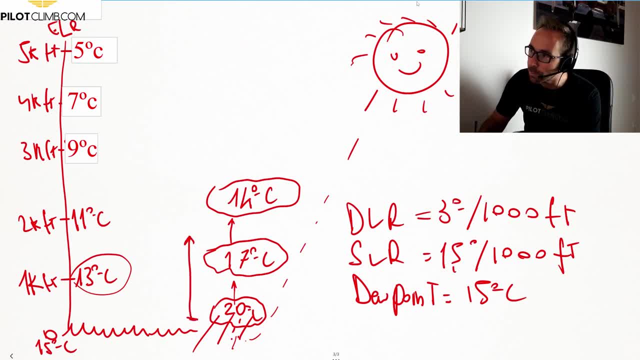 Thus, from here to there, let's call it in here, which is 15 degrees check mark, OK, From here to there, the mass of air, since it was not condensate, it was not saturated, it climbed using the dry lapse rate, OK. 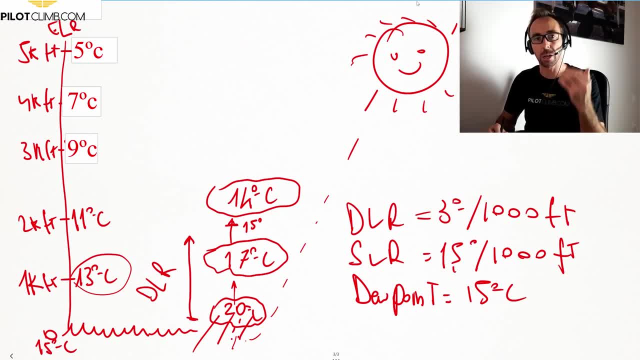 So the temperature: It was decreasing by 3 degrees every 1,000 feet. But once it reached the dew point, at 15 degrees, the mass of air start to condensate. So in this case we've got actually a cloud there, OK, And since we've got a cloud, what will happen is that, from this moment on, the temperature will decrease following the saturated lapse rate, which is 1.5 degrees every 1,000 feet. Thus, from this point, it will reach the. 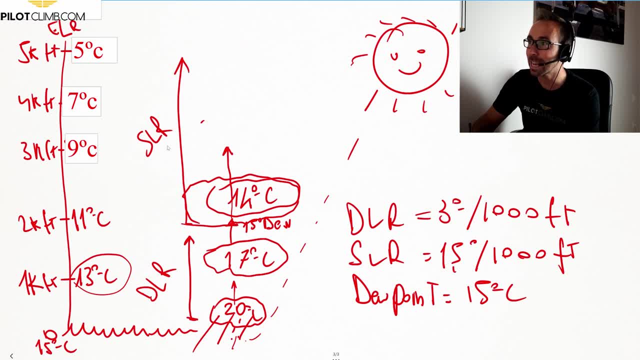 3,000 feet check mark. OK, As a cloud. OK, Because you have to imagine this is a cloud now, because it actually gets the dew point. and now it's a cloud. it's climbing as a cloud, Not anymore like as a mass of air. 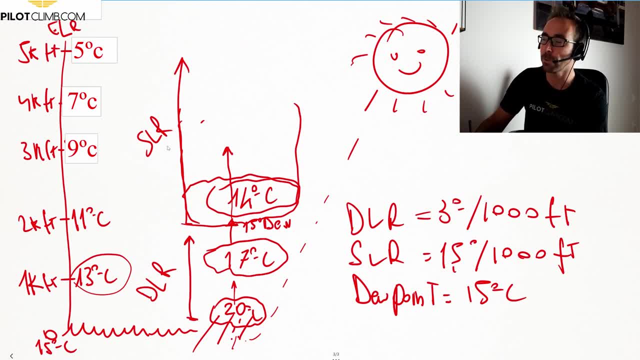 It will be from. it will pass from being 14 degrees, it will have 1,000 feet above. It's going to have a temperature of how much is it? 12.5 degrees, OK, Thus it's still, as you can see, it's still warm. 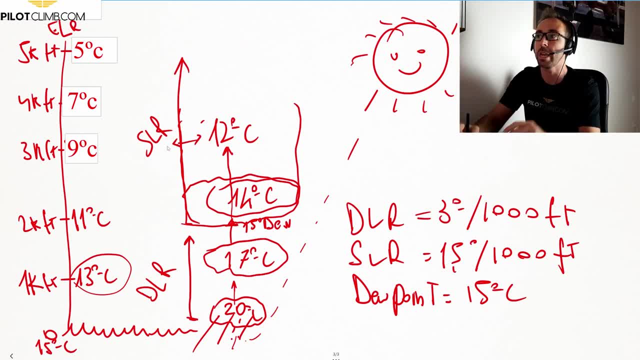 OK, The cloud at that altitude is still warmer compared to the outside, to the environmental air. Thus it's going to get to the 4,000 feet in here and it's going to have another 1.5 degrees less and will have. 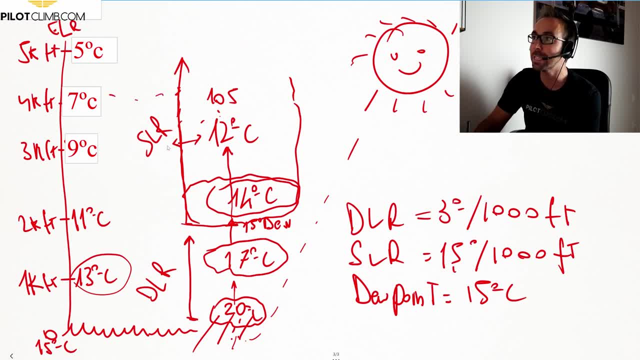 10.5 degrees at this check mark. OK, Thus, it's still warmer, guys. So what will happen is that the cloud will keep going, OK, And thus, and thus, as you can see, we have a change in the lapse rate. 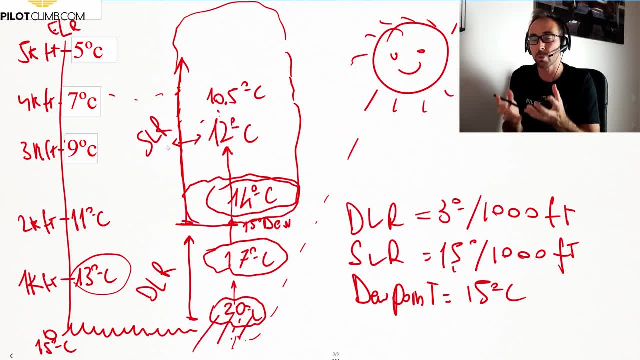 The dry adiabatic lapse rate is when the air must start to rise because it's lighter and warmer Since it's not saturated. OK, it will decrease with 3 degrees per 1,000 feet Once it gets becomes a cloud, because it